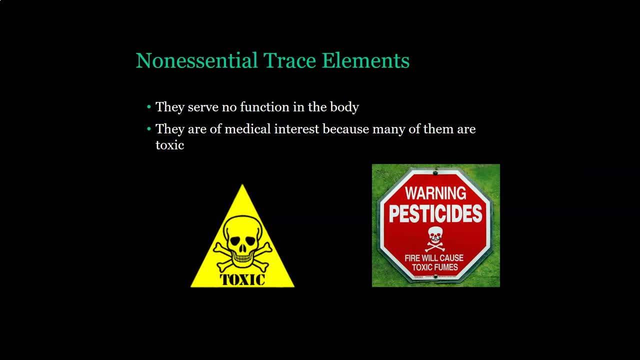 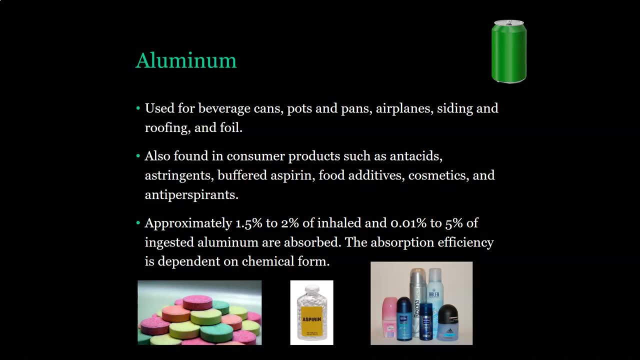 body, but they are of medical interest because many of them are toxic. Aluminum is used to make beverage cans, pots and pans, airplanes, siding, and roofing and foil. It is also found in consumer products such as antacids, astringents, buttered aspirin, food additives, cosmetics and. 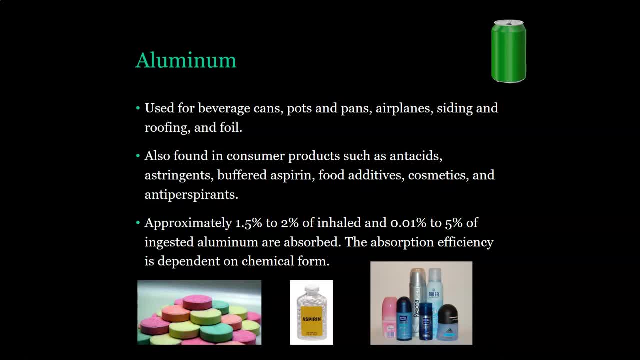 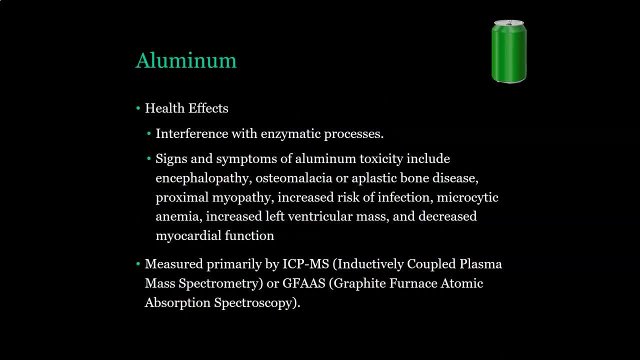 is approximately 1.5 to 2 percent of the inhaled aluminum is absorbed. The absorption efficiency is approximately 1.5 to 2 percent of the inhaled aluminum is absorbed. The absorption efficiency- chemical form. the health effects is that it interferes with enzymatic processes. 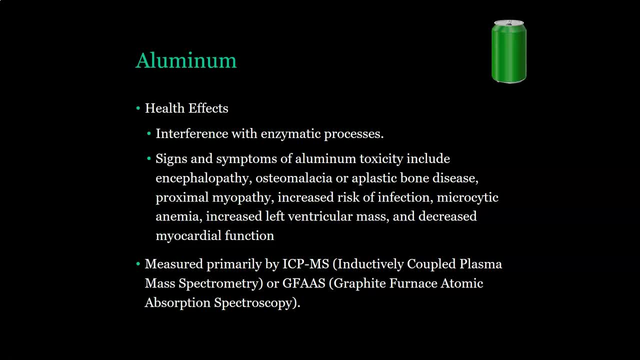 signs and symptoms of aluminum toxicity will include encephalopathy, osteomalacia or aplastic bone disease, proximal myopathy, increased risk of infection, microcytic anemia, increased left ventricular mass and decreased myocardial function. it is measured probably primarily by acpms, inductively coupled plasma mass spectrometry and graphite furnace atomic. 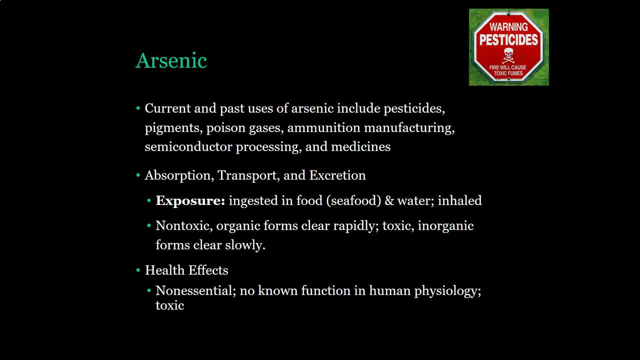 absorption spectroscopy. arsenic. current and past uses of arsenic include pesticides, pigments, poison gases, ammunition manufacturing, semiconductor processing and medicines, including some treatments for leukemia. the exposure it will be: it can be ingested in food, in seafood and in water and can also be inhaled. exposure. the non-toxic organic forms of arsenic will clear. 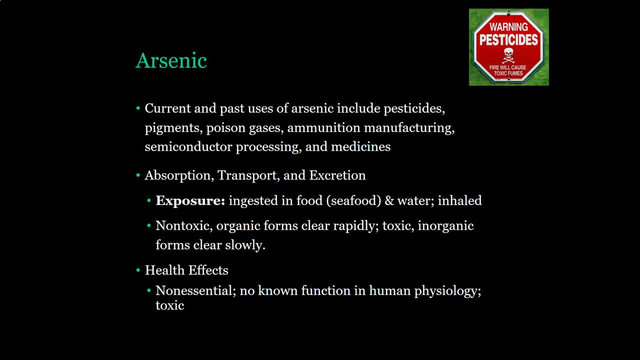 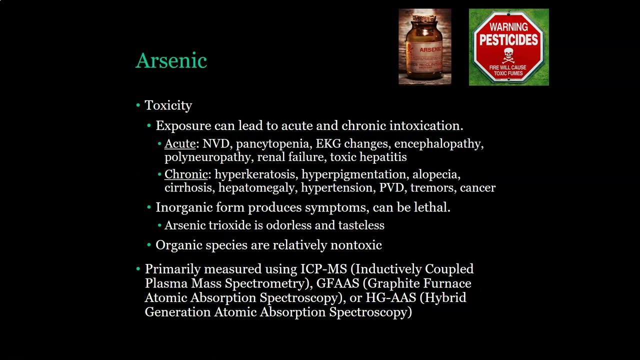 rapidly, but the toxic inorganic forms will clear slowly and cause problems. it is non-essential mineral, it has no known function in human physiology and it can be toxic. the toxicity so exposure can lead to either acute or chronic intoxication depending on the type of exposure. 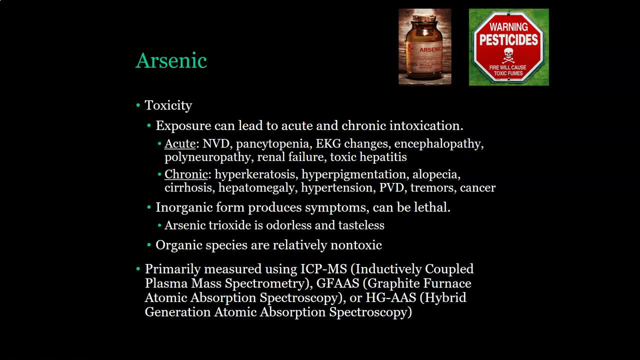 um. acute intoxication signs and symptoms will be not a vomiting diarrhea with abdominal pain and stuff hand cytopenia, so like bone marrow depression, ekg changes, encephalopathy, polyneuropathy, renal failure, toxic hepatitis. chronic forms are going to be hyperkeratosis, hyperpigmentation. 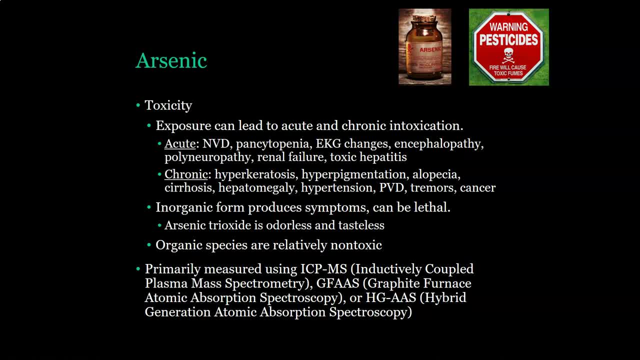 alopecia, cirrhosis, hepatometaly, hypertension, peripheral vascular disease, tremors and cancer. so that's all with chronic uh. exposure to arsenic, the uh inorganic form, produces symptoms, uh and it can be lethal. and arsenic trioxide is odorless and tasteless and that's often the poison. 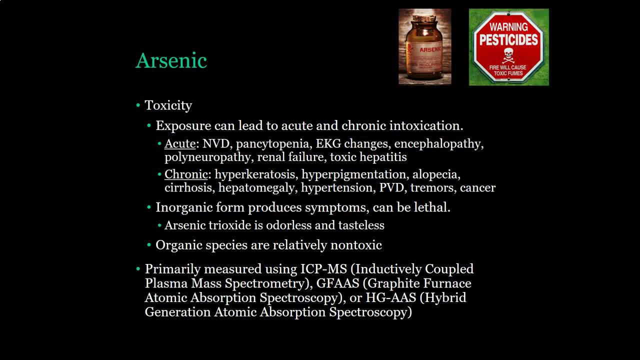 use that can be used to kill people. uh, the organic species of arsenic are relatively non-toxic and easily cleared by the body, and is primarily measured using icpms and graphite furnace, AAS and, but then also hybrid generation, atomic absorption, spectroscopy, cadmium. 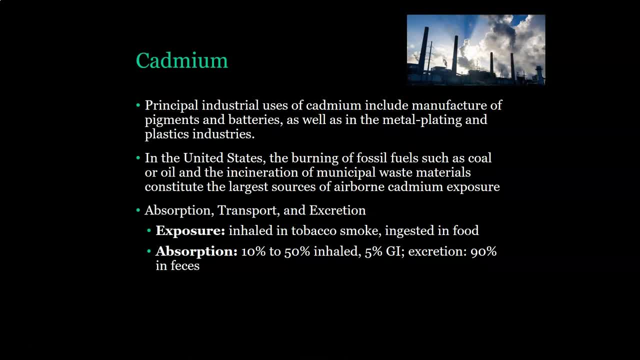 the principal industrial uses of cadmium include the manufacture of pigments and batteries, as well as metal plating and plastic industries. in the US, the burning of fossil fuels such as coal or oil and the incineration of municipal waste materials will constitute a large source of airborne cadmium exposure. 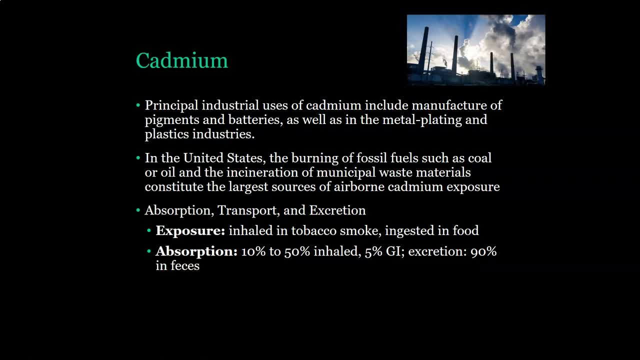 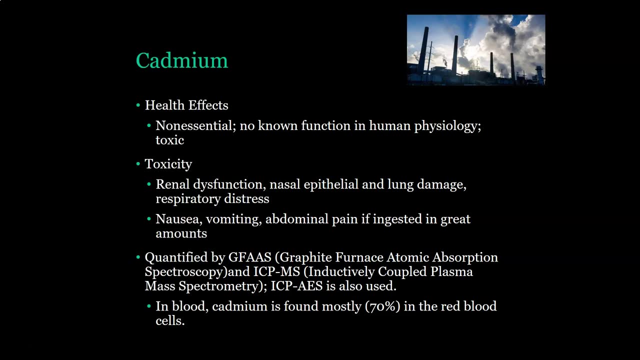 it is inhaled in tobacco smoke and ingested in food. you will absorb 10 to 50 percent of what is inhale and 5 percent of what is ingested, and you excrete 90 percent of it in feces. the health effects: this is obviously not essential. 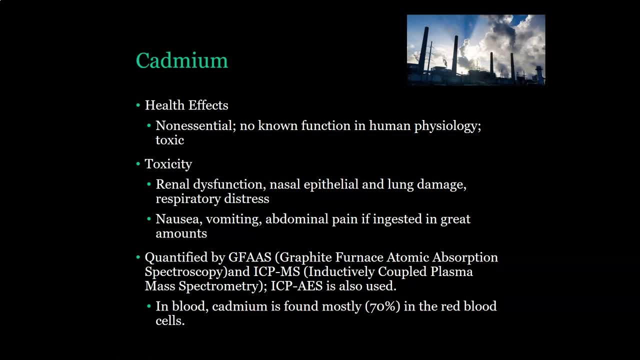 no known function and is toxic toxicity, you will see renal dysfunction, nasal, epithelial and lung damage and respiratory distress. obviously, if it's inhaled and ingested, nausea, vomiting, abdominal pain. but you have to ingest pretty significant amounts. it is quantified by graphite furnace, AAS and ICP-MS and it 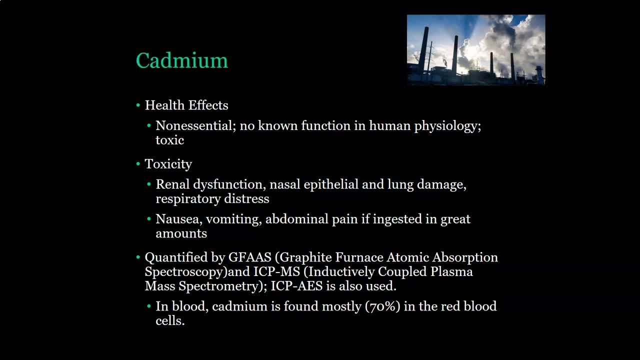 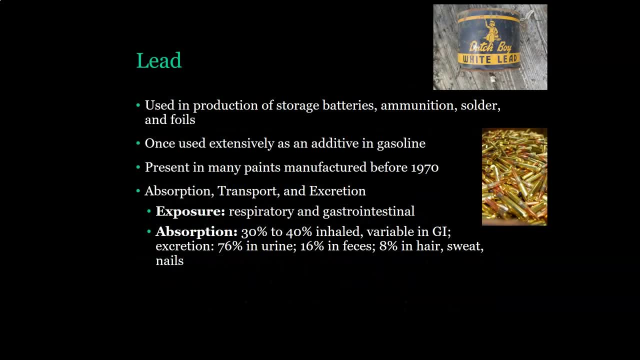 can also use ICP-AES in blood. cadmium is found mostly in the red cells, increased in the red cells, so you would want to do a whole blood analysis. lead is used in the production of storage batteries, ammunition, solder and oils. it was once used extensively as an additive in gasoline and it was present. 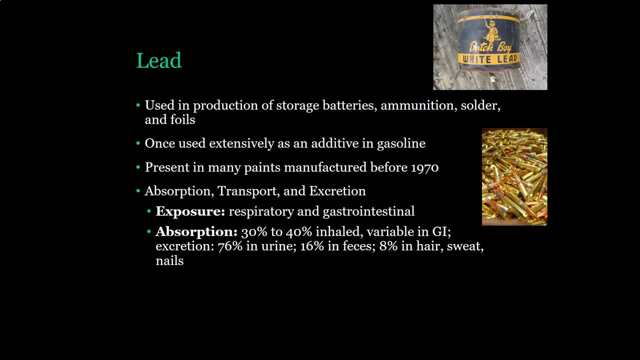 in many paints that were manufactured before 1970, so it can be in like old houses and stuff. the exposure to lead can be a VI, respiratory or GI system. you will absorb 30 to 40 percent of what is inhaled and the absorption is variable. 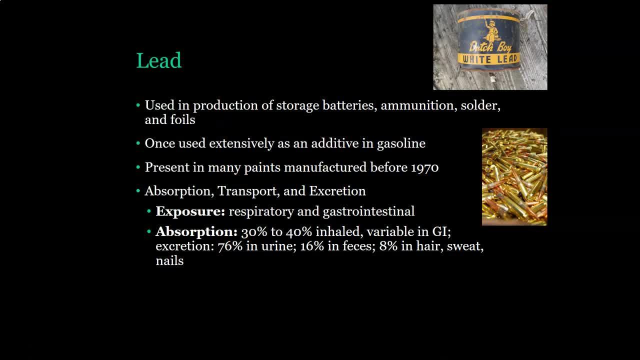 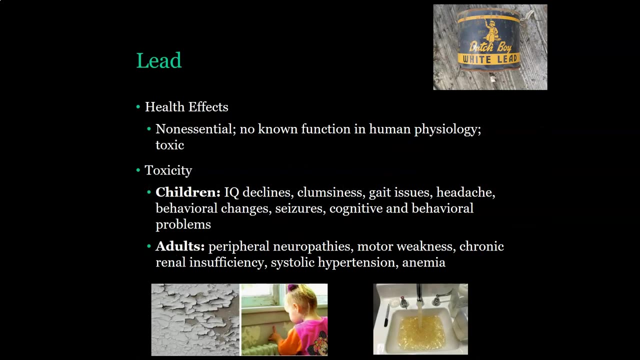 and the GI will depend on the status of your GI excretion. 70 percent- 70 percent of it is excreted in urine, 16 percent in feces and eight percent in hair sweat and nails. the health effects is obviously. it's non-essential and it doesn't have any function and it's actually 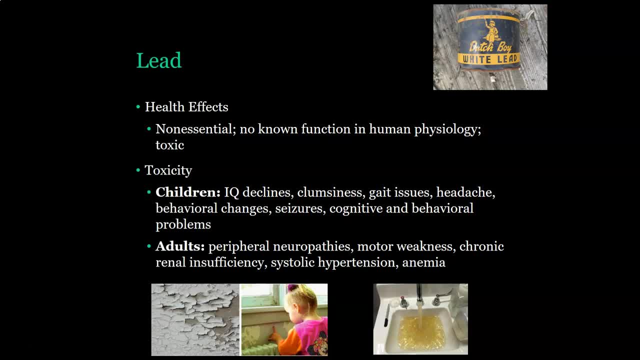 toxic. the toxicity in children. you will see IQ declines, clumsiness, gait issues, headache, behavioral changes that are like bad ones, like negative ones, tantrums, fits and all that seizures um cognitive and behavioral problems. in adults, you will see peripheral Neuropathies, motor weakness, chronic. 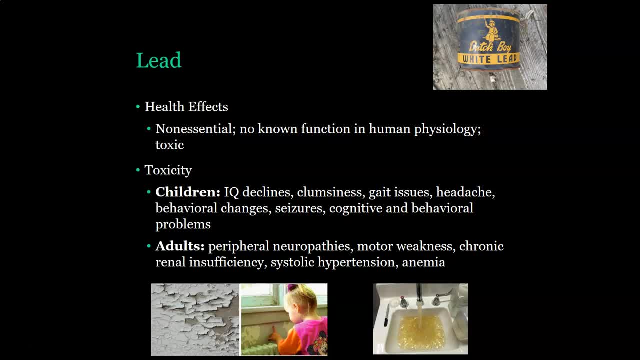 renal insufficiency, systolic hypertension and anemia and um. so you see here in old paints and stuff- and kids tend to put old paint chips in their their mouths and stuff- but uh, the Flint Michigan water crisis when they switched their water source and it was contaminated, so they 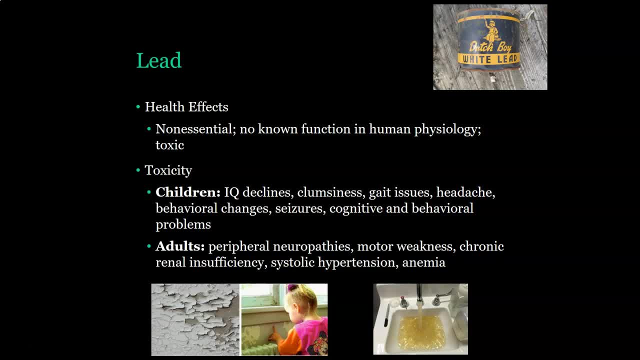 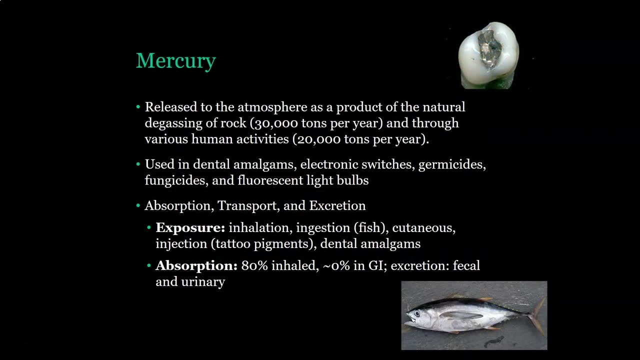 increased the chlorination of the water and the uh that caused the leaching of from lead pipes. and then you have brown water that was full of lead and then you end up with lead poisoning in children and adults. Mercury: it is released into the atmosphere as a product. 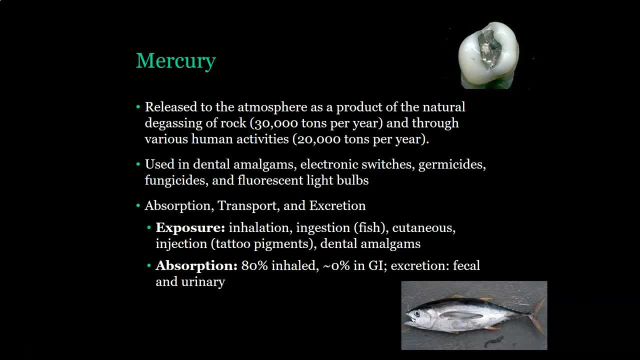 of the natural degassing of rocks and through various human activities. It is used in dental amalgams. so your silver fillings, electronic switches, germicides, fungicides and fluorescent light bulbs. Exposure is through inhalation or ingestion, especially ingestion of fish like